The area which appears two at a spot is called the V-be degnation. The dengan eye of the triangle is marked by the side that derives an angle letter. The line dictates for it whether the sides are corresponding or converging or inclinating to the angle. 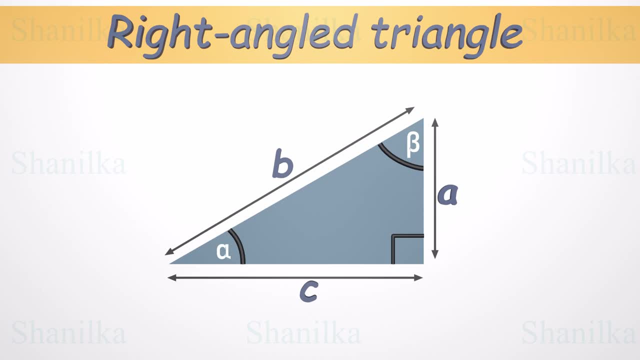 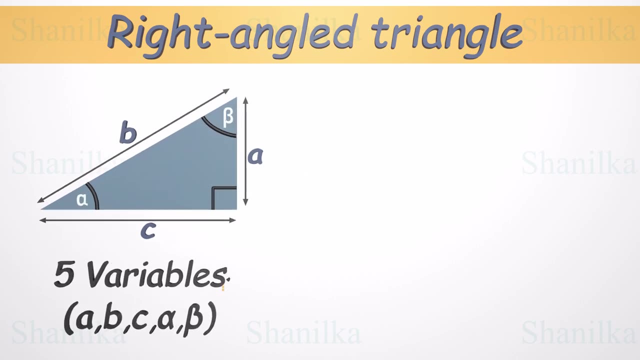 Knowing how to accurately label the sides for a specific reference angle is essential. As I mentioned earlier, the simplest geometric shape with only has three sides and three angles. In right angled triangles, we surely know, one is always a right angle. So there are five unknowns. If we know any two of, 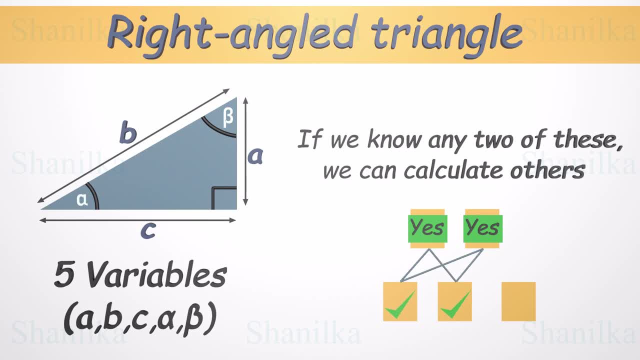 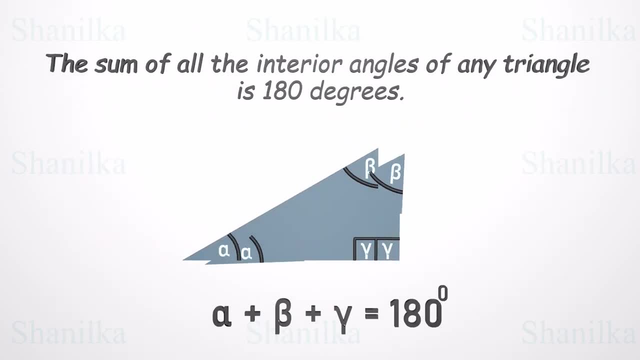 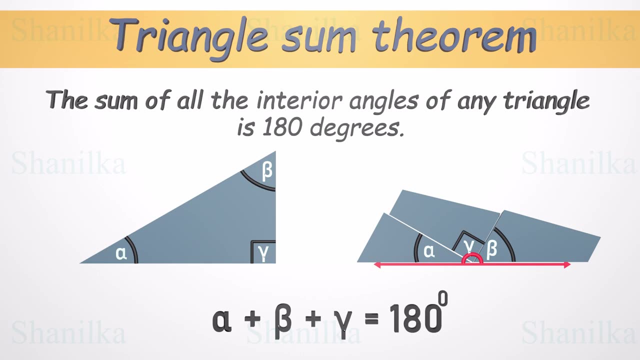 these. we can calculate others using the knowledge of trigonometry. Before going further, we have to brush up on our knowledge of geometry. The first one is that the sum of all the interior angles of a triangle is 180 degrees. We call this the triangle sum theorem. So if we consider two, 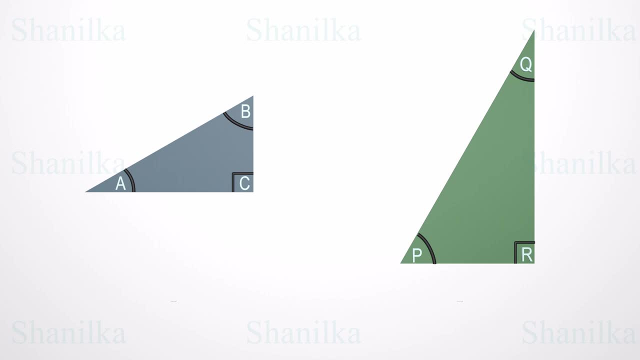 right angled triangles. the sum of the interior angles of each triangle is equal to 180 degrees, And we already know that in right angled triangles one angle is always 90 degrees. So the sum of the rest two angles is also equal to 90 degrees. 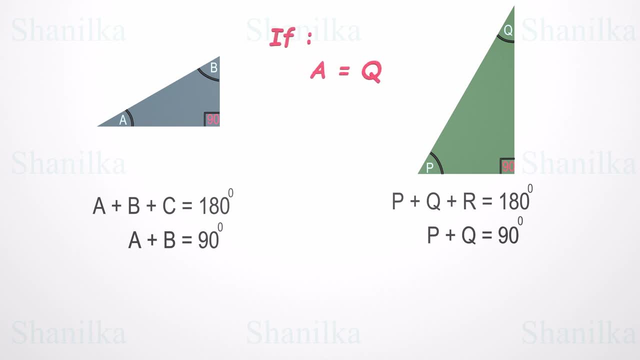 Now assume the angles A and Q are also equal. Let's say those are equal to alpha degrees. Then both B and P are equal to 90 minus alpha. Let's say it's equivalent to beta degrees. Now we can see in both triangles the corresponding angles are equal to each other. 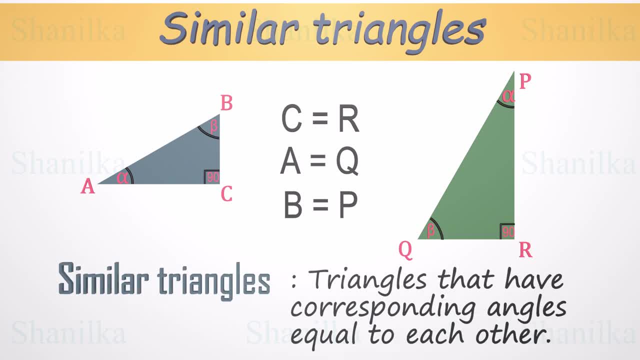 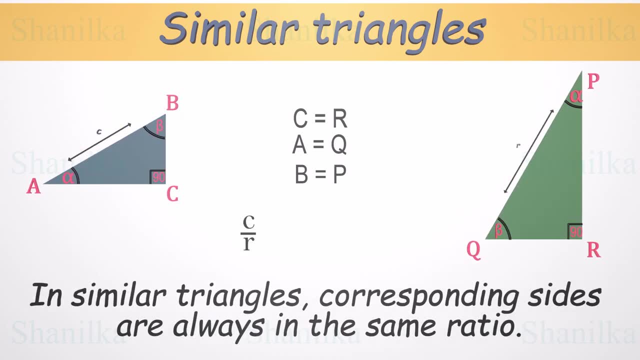 So those are similar triangles. Early mathematicians have identified that in similar triangles, corresponding sides are always in the same ratio, And so the ratio of the sides of a triangle is the ratio between two sides of a triangle. The relationship between the sides of a triangle and the side of a triangle is equal to one. 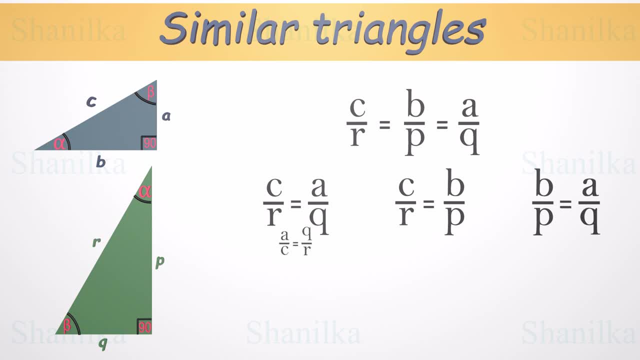 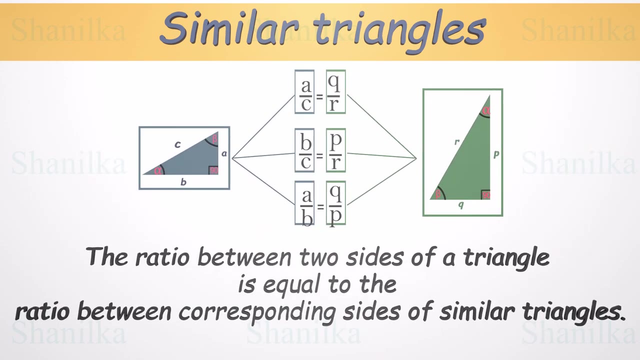 Now we have a relationship between two similar right angled triangles. This relationship can be separated into three parts. Let's rearrange these three equations. Are you with me up to this point? So let's clear the rest and keep our last equations: corresponding sides of similar triangles. This is very useful. It is the foundation. 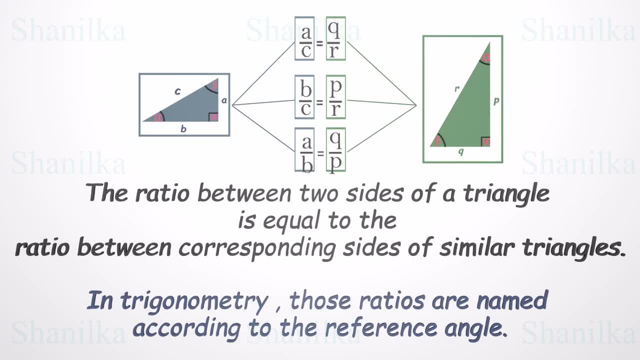 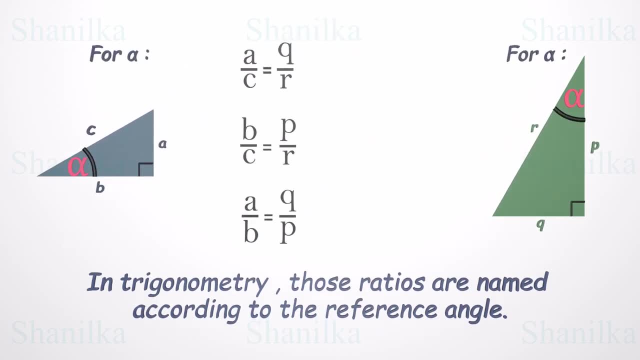 of trigonometry. So in trigonometry we name those ratios according to the reference angle. Let's consider the angle alpha as our reference angle. C and R are hypotenuses. A and Q are opposite sides for angle alpha. P and B are adjacent sides for angle alpha. 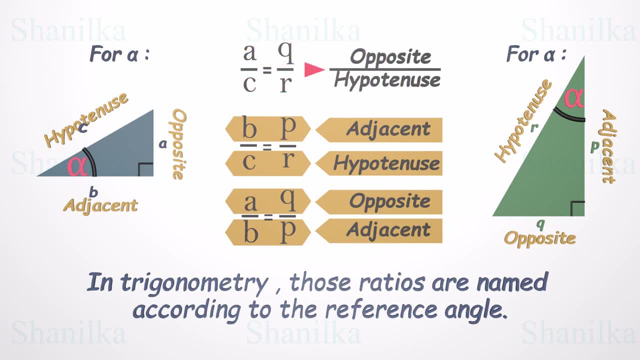 So the first relationship is the ratio between the opposite and hypotenuse of the alpha angle. The second relationship is the ratio between the adjacent and hypotenuse of the alpha angle. The third relationship is the ratio between the opposite and adjacent of the alpha angle. 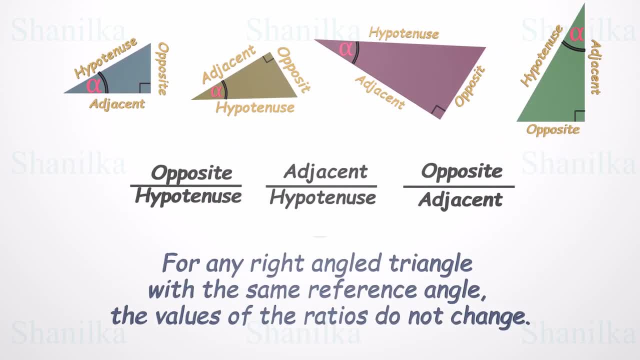 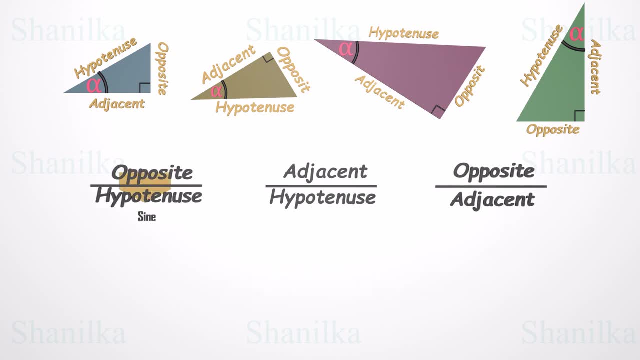 of a right-angled triangle. For any right-angled triangle with the same reference angle, the values of the ratios do not change. We named those sine cosine and tan To indicate the reference angle. we wrote those like this: Those are the three fundamental trigonometric ratios. 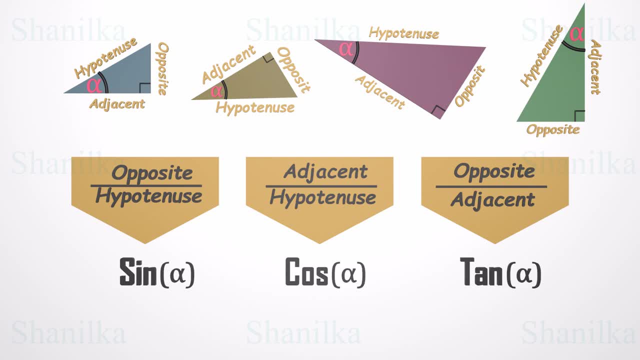 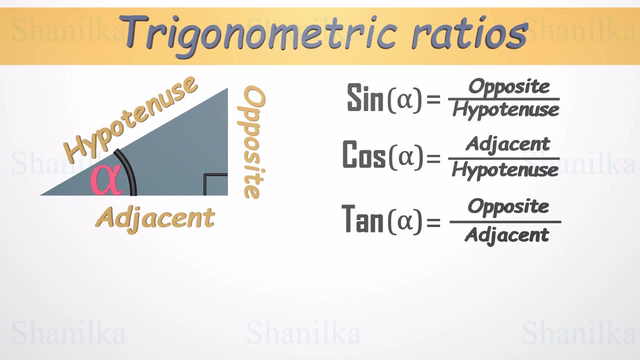 So next time someone mentions a sine cosine or tan, don't be afraid They are talking about the ratio between two sides of a right-angled triangle in reference to an angle For any particular angle. there is a constant values for these ratios. 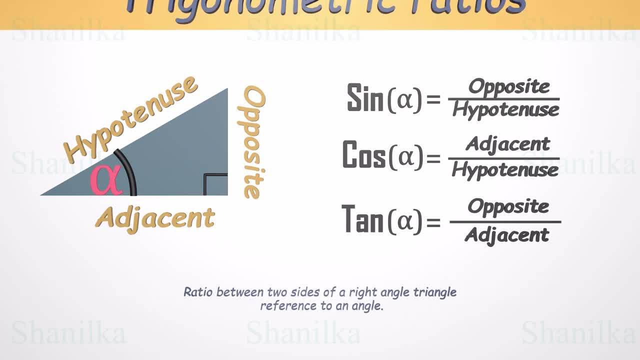 For example, if we want to know the angle of the right-angled triangle, we can write the angle of the right-angled triangle as the angle of the right-angled triangle. We can write the angle of the right-angled triangle as the angle of the right-angled triangle. 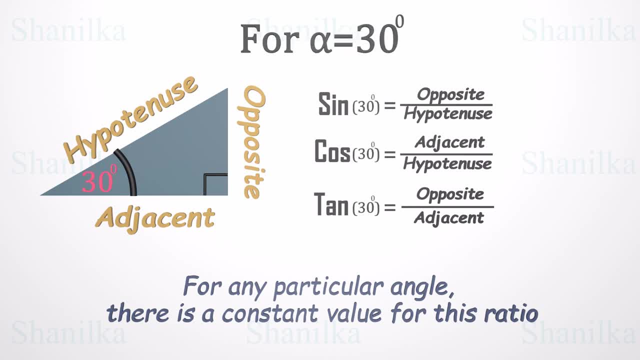 For example, let's consider the angle as equal to 30 degrees. For the sine ratio, we get 0.5.. For the cos ratio, we get 0.866.. For the tan ratio, we get 0.577.. 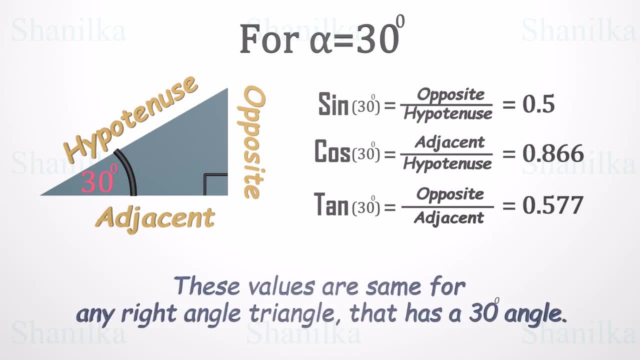 These values are the same for any right-angled triangle with a 30-degree angle, No matter what the size and orientation are. If we consider the alpha as 45 degrees, For the sine ratio, we get 0.707.. For the cos ratio, we get 0.7072.. 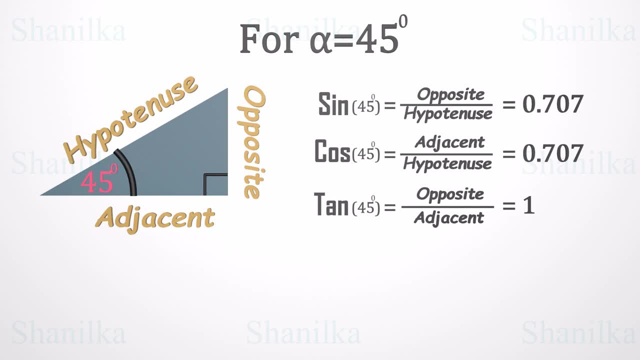 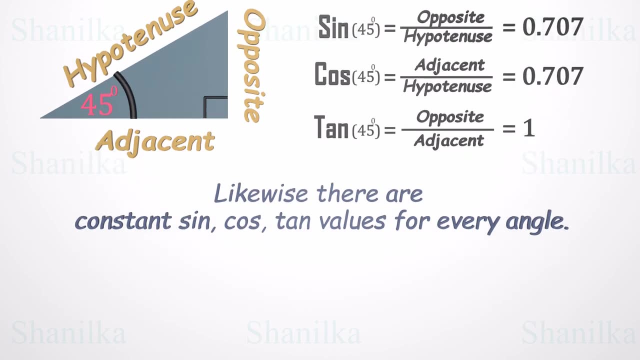 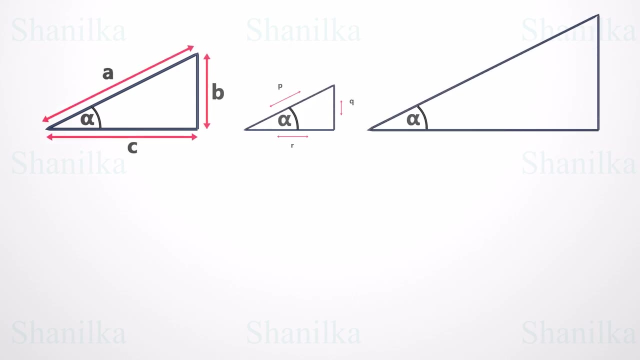 For the tan ratio, we get 1.. Likewise, every angle has constant sine, cos and tan values. If you have any doubt about this, please try to draw several triangles at different sizes but with the same angles, Then measure the lengths and calculate the ratios of the corresponding sides of each triangle. 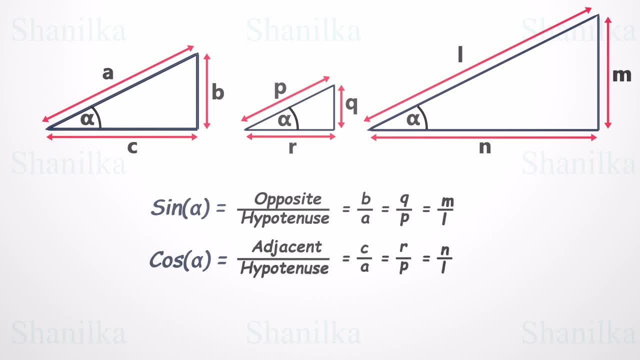 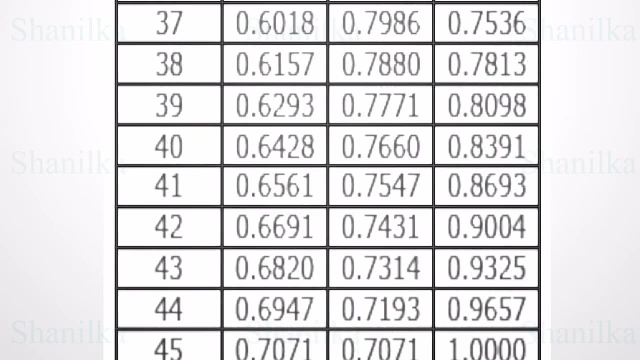 Each triangle will get the constant sine, cos and tan values common to every angle, But we don't have to measure the sides and calculate these ratios every time we need them. There are pre-calculated value tables for those, and most of our calculators come with trigonometric functions.